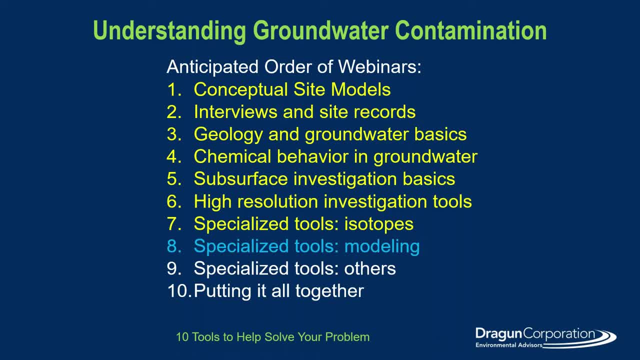 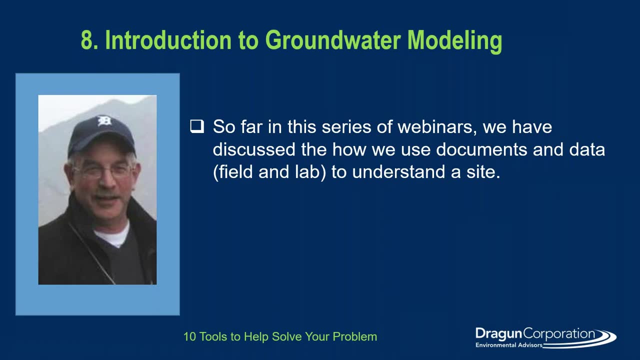 contamination. The yellow ones are ones we've already done, and today's is on modelings in blue. So far in the series of webinars, we have discussed how we use documents and data, that is, field and lab data, to understand a site. The groundwater modeling part combines this information. 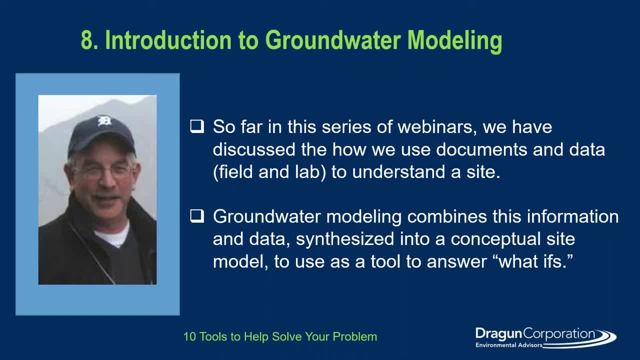 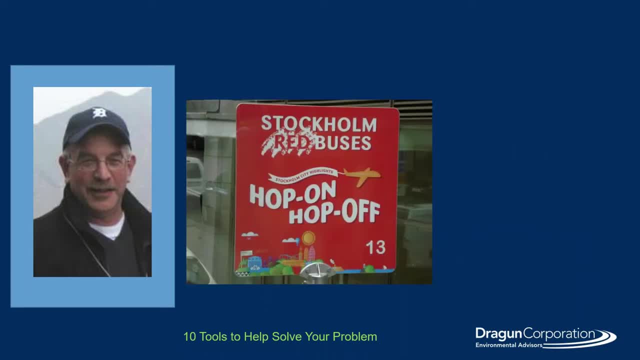 and data. It synthesizes it into a conceptual site model and we use that as a tool to answer what-if questions. So I'd like to take a moment here and allow you to keep going, or keep with us on this. You'll not learn how to run a groundwater model here today. However, you may learn something. 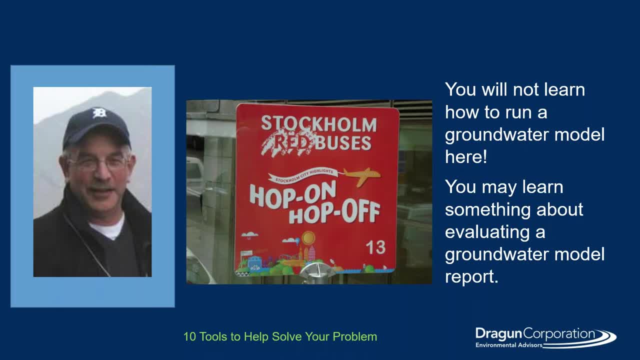 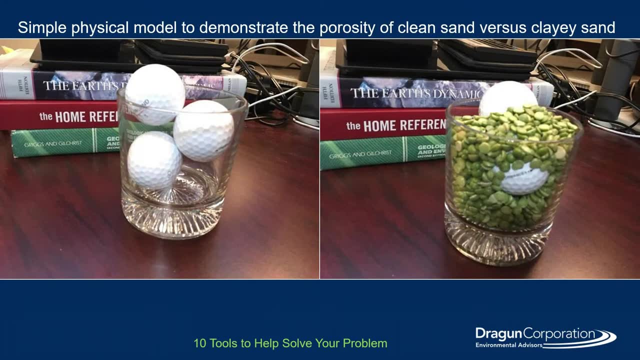 about evaluating a groundwater model report You may find on the right hand side to the right itvект neighborhood or university website. it's called the community webinar. so it's gonna be a fun littleEEP debate and we'll see where you guys try to lean in on those. 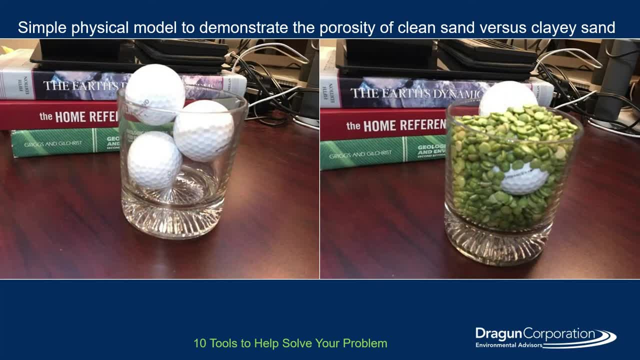 Great. So, as we relate to hand равonder modeling, we're looking at different models. So you've by split peas. So a simple model is good if it brings about a meaningful understanding of a problem. Today, our main topics will be: what is the? 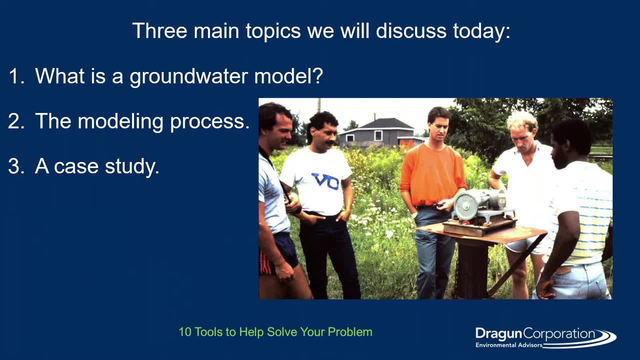 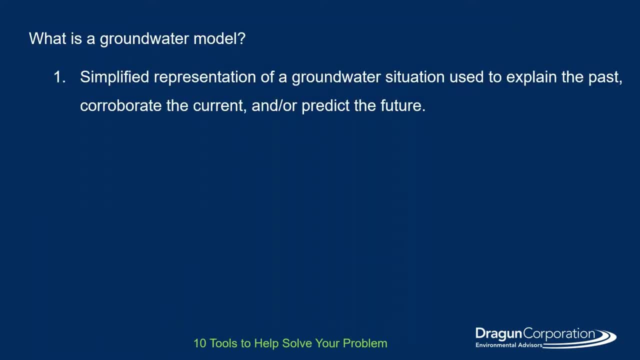 groundwater model. what's the groundwater modeling process? and we'll use a real case study to help with explaining the modeling process. So what is the groundwater model? Groundwater model is a simplified representation of a groundwater situation used to explain the past, corroborate the current and or 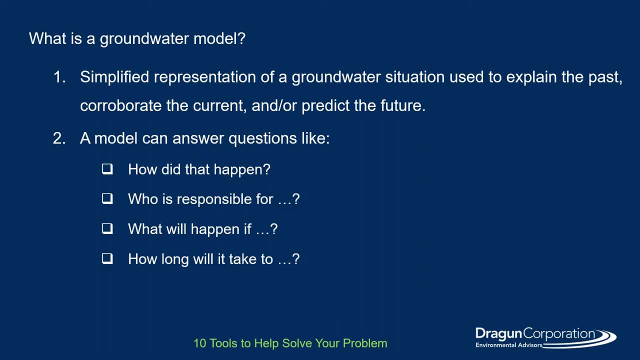 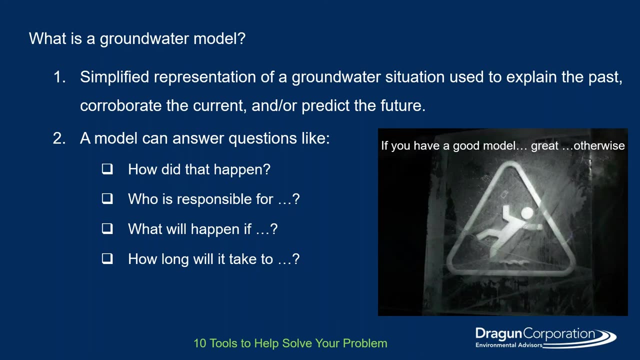 predict the future And a model can answer questions like: how did that happen, who's responsible for this, what will happen if we, and how long will it take to? And if you have a good model, you'll get answers to these questions that you can use. That'd be great. otherwise, you're in trouble. So what is? 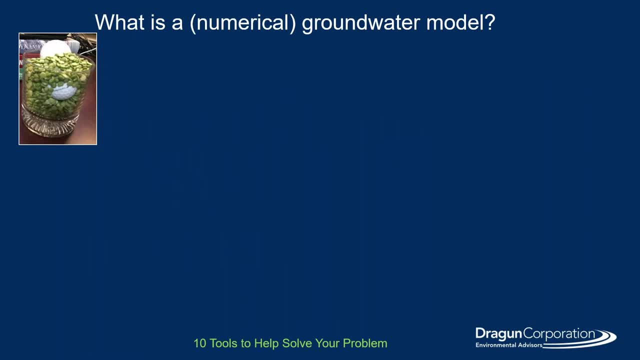 a numerical model, A numerical groundwater model. Groundwater model can be as easy as an equation. This is the Tice equation that's used for evaluating well responses to pumping. That's been around and in use since the 1930s, I believe. 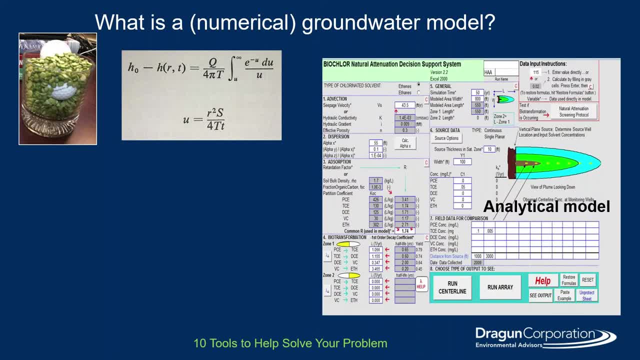 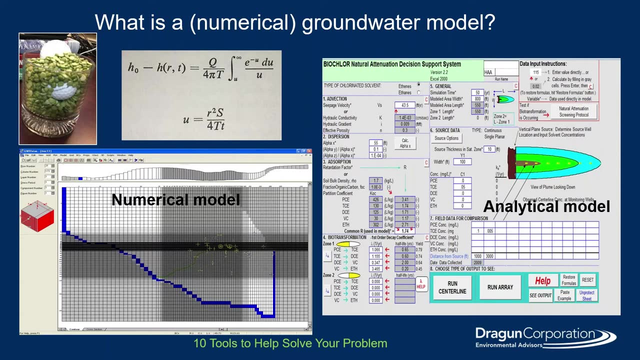 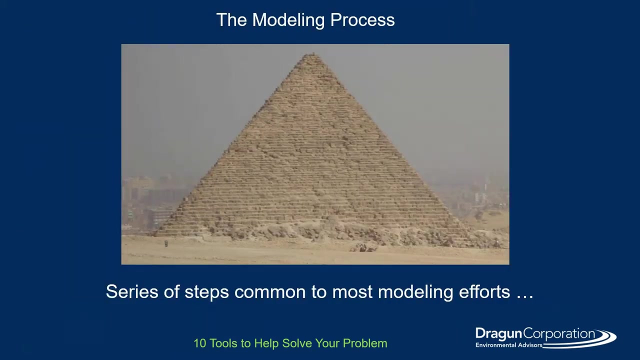 An analytical model is one that can be used to solve simple problems with equations and often is used in a spreadsheet form. And then a numerical model is for more complex problems and requires specialized computer codes that distribute parameters throughout the modeled area. So these are the modeling steps you need to look at when you're reviewing a model. 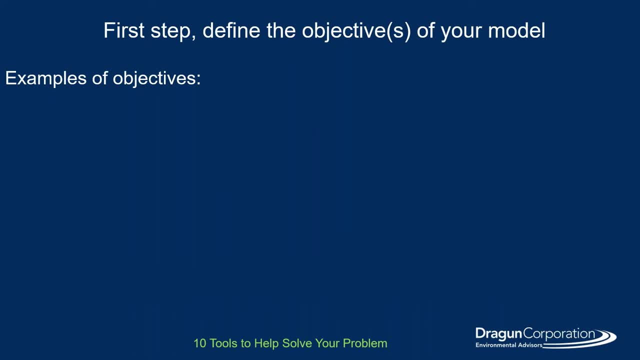 First step is to find the objectives of your model. There are lots of different things you can do. You can say with you know, if you're looking at a water supply, if we add another well, will that be enough to supply the community without causing problems? If we add another well, will we dry out a stream? 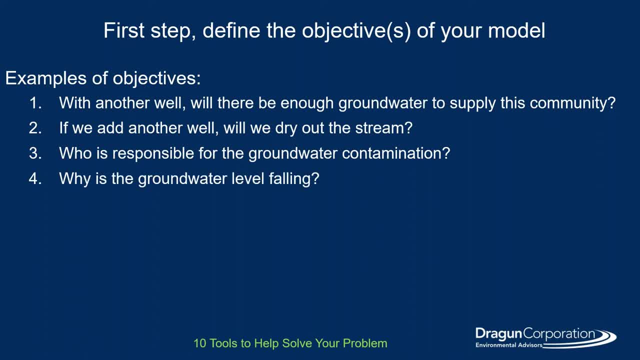 Who's responsible for the groundwater contamination? Why is the groundwater level falling? Are there enough wells to capture the contamination through? When will the contamination reach the wells? What will concentration be at a well in 30 minutes? What will concentration be at a well in 30 minutes? What will concentration be at a well in 30 minutes? 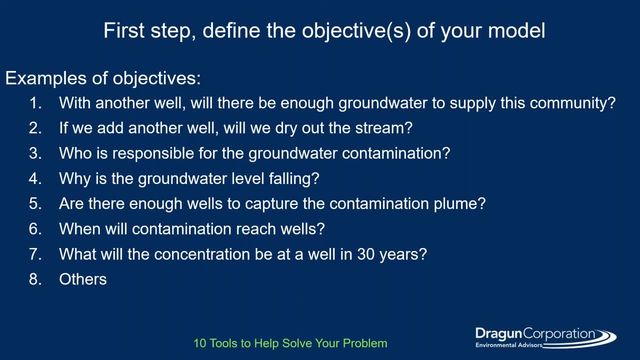 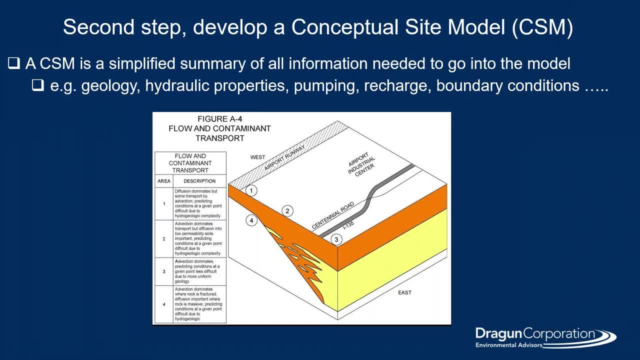 And there's all sorts of other things that you can pose as questions for the model. The second step is develop a conceptual site model. This is very important because it takes all the data and information you have and summarizes, for example, the geology, the hydraulic. 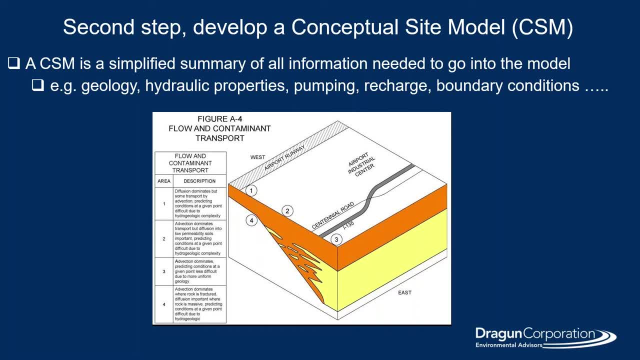 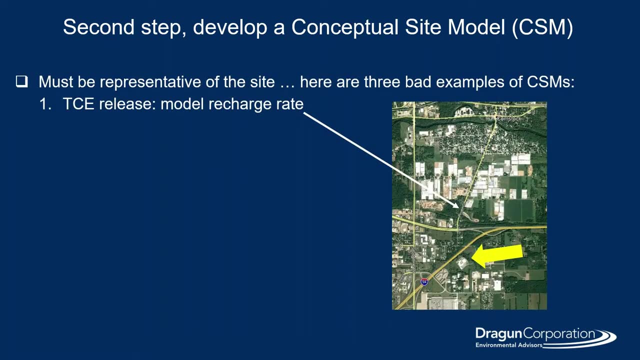 properties, how water can move through soil and rock, pumping, recharge, boundary conditions. Models have spatial limitations, So the edges, soil, the water and the water and water conditions are very important. Your model depends to a great deal on how good your conceptual model is. 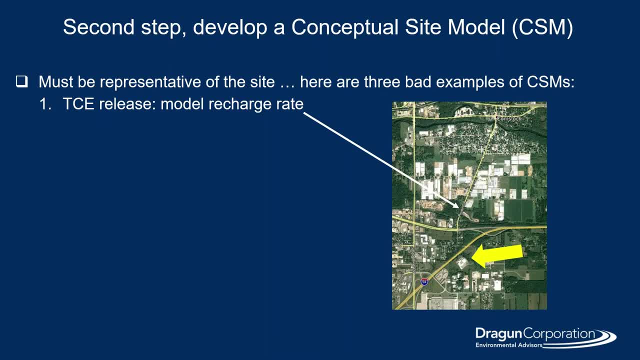 Over the years I've ran into a number of bad examples. This first one is a site that I worked on where somebody had created a model where there was released from a manufacturing facility at the tip of the yellow arrow- and that was a TCE release- and the groundwater is flowing from bottom to top and they wanted to. 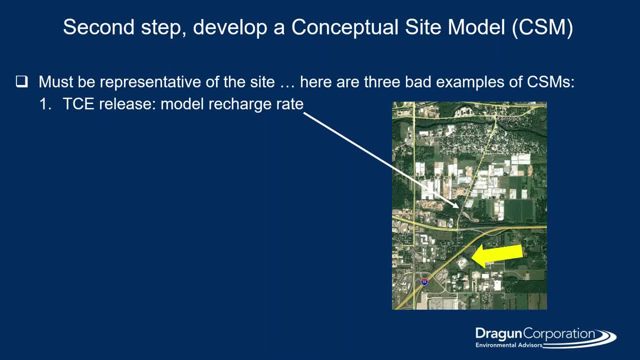 evaluate how to clean this site up. Well, they used a one factor input in the model of recharge, which is precipitation, some factor of precipitation, and they used the snowfall equivalent or they did not use the snowfall equivalent for snowfall. That means they were. 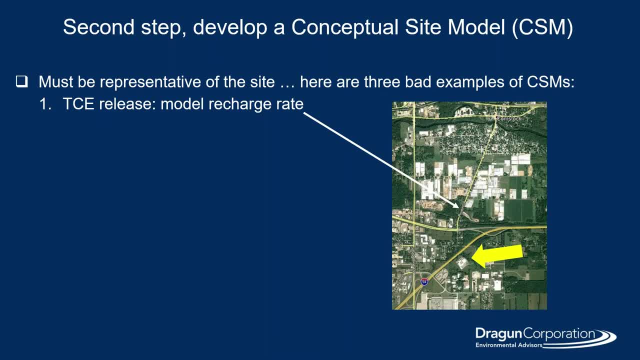 off by about 10 times, and that affects all the other parameters in your model, so that didn't work out too well. This next one is another one. well, really, the first project I worked on is the consultant. There are two landfills at the tips of the arrows here. 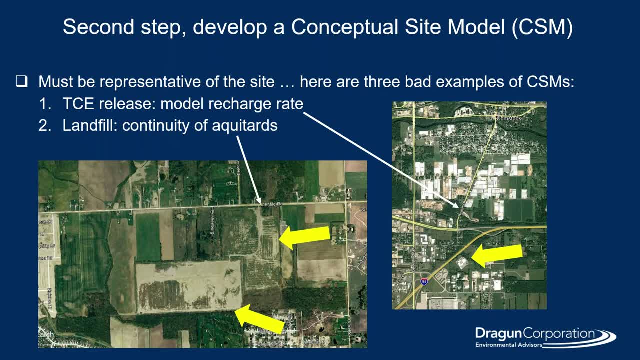 and the regulators assumed that there were holes in the aquitard or the clayey soil under the landfill on the north side- the top yellow arrow- And they did that in their model in a lawsuit and there was no field data to support that. 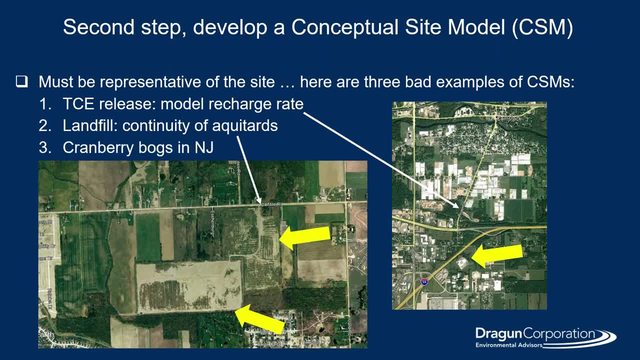 We actually went out and showed that to them And then, finally, I don't have a figure for this, but worked on a project early in my career on the cranberry bogs in New Jersey And there was TCE in the groundwater and they wanted to look at how far the ground TCE would go. 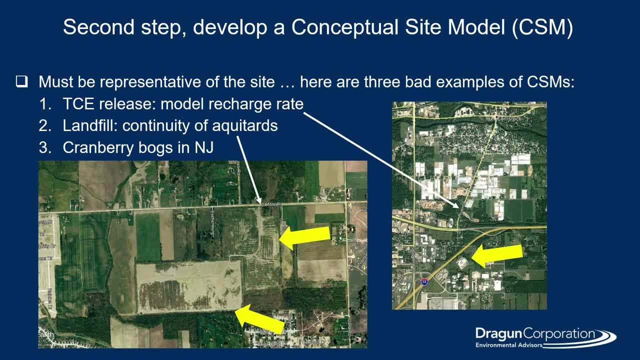 And the model that was being used showed that it all ended up in a cranberry bog. Well, when they went and got field data beyond the cranberry bog, they found TCE. So again, if the model doesn't fit the observations, it's not a good conceptual site. 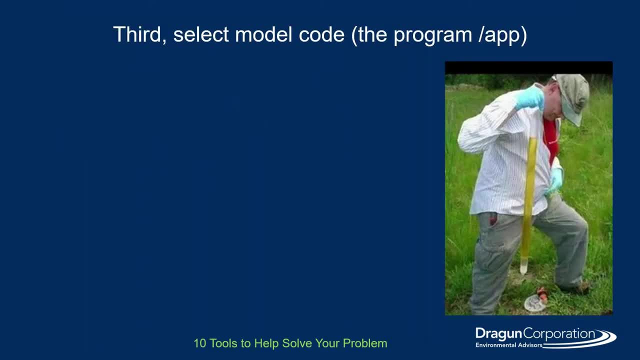 Slide 22. So the third thing you need to do is select the model code. There's lots of questions to consider here. Is it groundwater flow, where you say you might just want to know about water levels, or flow and transport Do you want to know about? 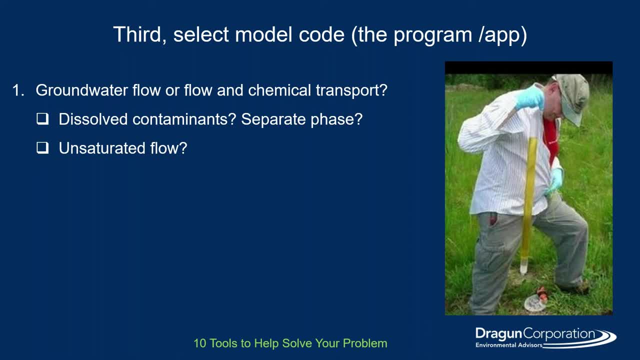 how far contaminants will move? Are you looking at dissolved contaminants or separate phase, like we see in this picture, Or are you looking at unsaturated flow above the water table? Slide 23: How do you want to simulate dissolved chemical movement? The easiest is advection. That's the 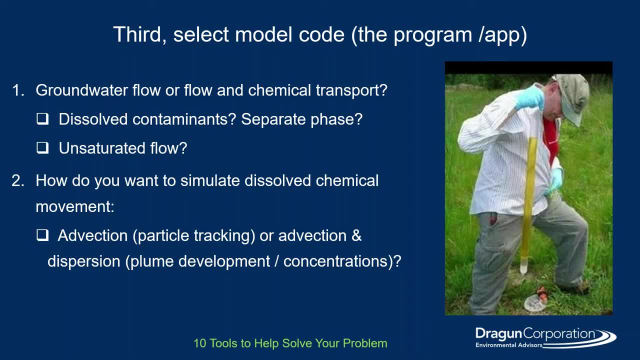 way that particles are just moving with the groundwater flow And we use a particle tracking code for that. Or advection and dispersion, where you can actually see a plume develop in three dimensions and you can follow concentrations, But that's a much more intensive. 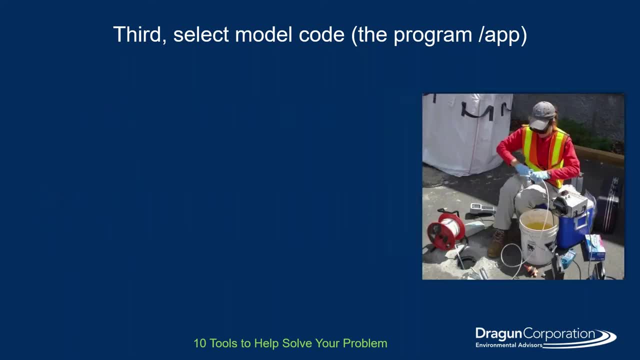 endeavor, Slide 24. So how many dimensions are important and why Do you have one dimension, two dimensions or three dimensions? The one we're going to show you later is a three-dimensional model where you're concerned about vertical variations in where the plume is. 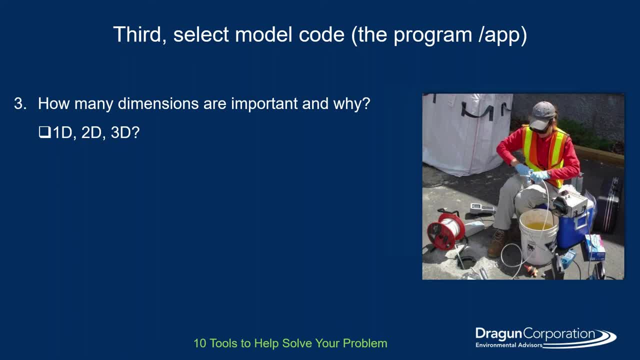 as well as aerial variations. But if the aquifer is thin, for example, you only need two dimensions. Slide 25: Is it steady state or transient? Do the factors in your model change with time, like does pumping start or change during the modeling period, Or are there changes in recharge rates that 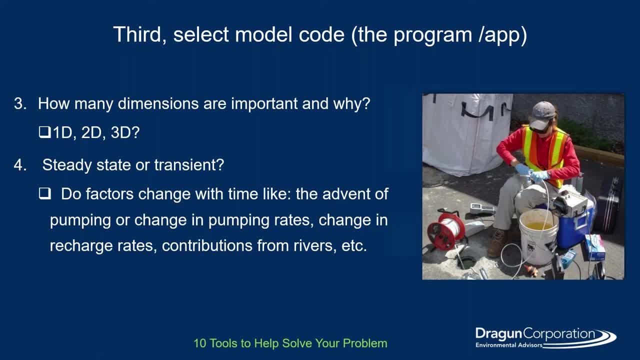 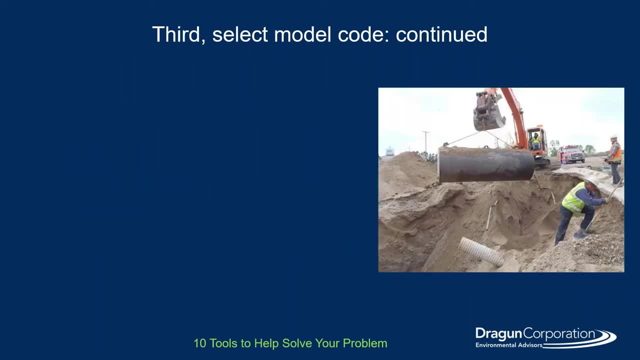 might come about by pavement, development, parking lots or contributions to rivers. Do they change with time? Slide 26. Slide 27: Do you want to use a numerical? Slide 28: Do you want to use a numerical or analytical code? Well, 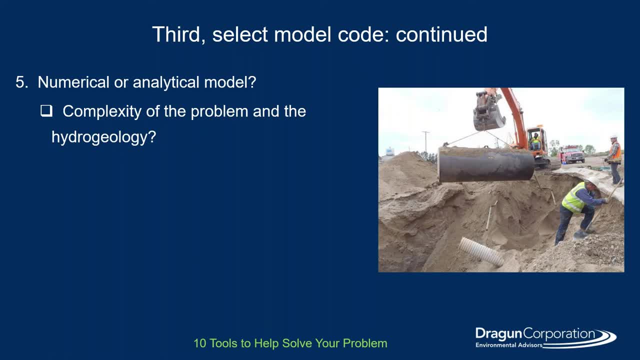 if you have uniform conditions in hydrogeology and time, an analytical model which is simpler might be useful, But if you have a complex problem, you probably want to go with a numerical model, Slide 30- And which product will serve you best? 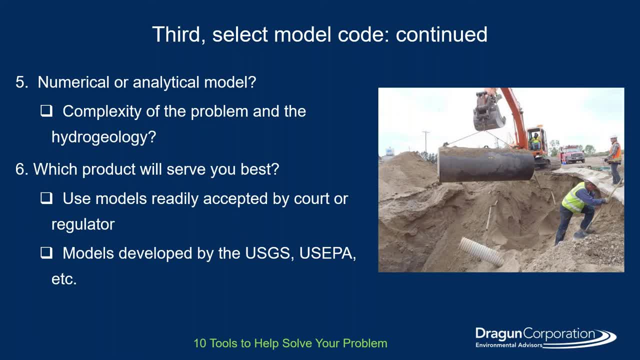 Slide 31. I like to use models that are readily acceptable by the court or the regulator, And some of these are the ones that are developed by the US Geological Survey and the US EPA, And that saves you the effort of having to defend. 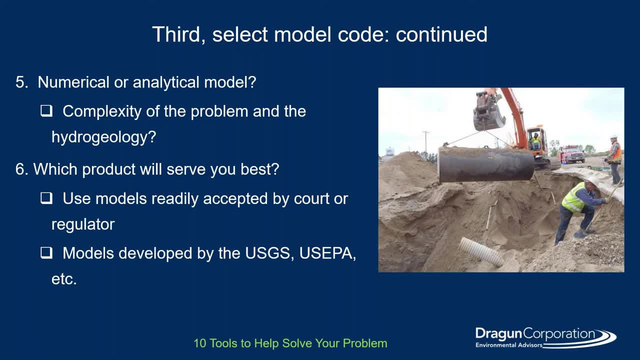 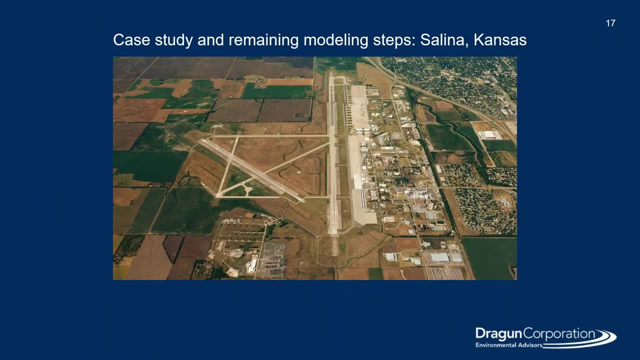 the model that you're using, the code that you use in your project, Slide 32. So we're going to look at a case study to go over the remaining modeling steps. And this is a site in Kansas. The town is Salina, Kansas, and it's a former 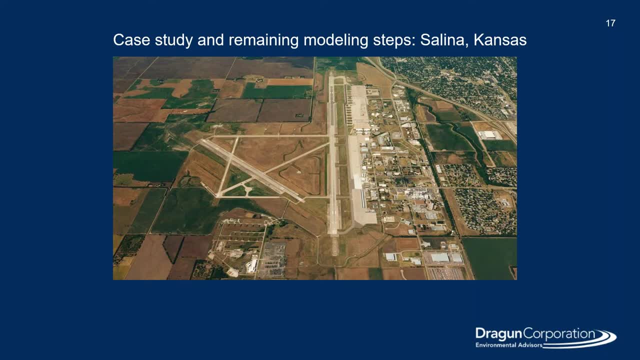 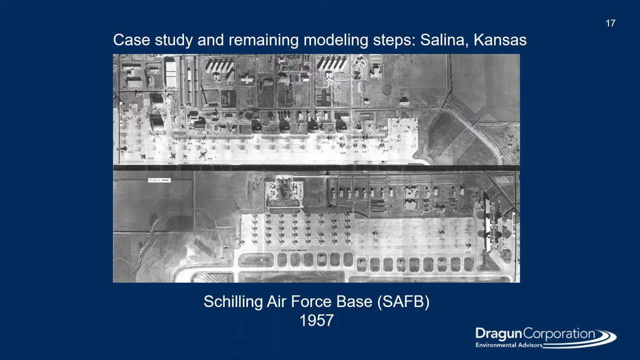 strategic air command base and air force base in the 1950s and 1960s mostly And they used lots of solvents and they used that to clean planes and also parts of planes. And there are 11 groundwater plumes, mostly TCE. There's some PCE and carbon tetra chloride- that this 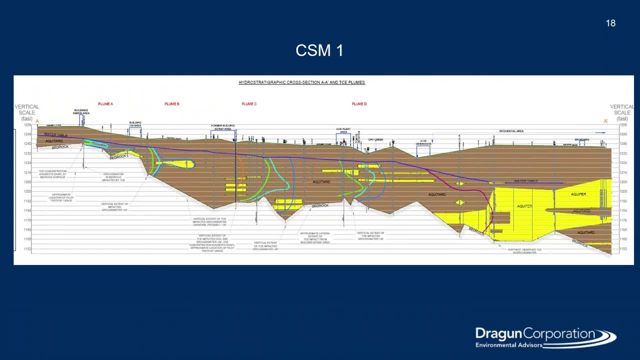 So when we were looking at this model, we were developing a conceptual site model, which involved things that we call hydrostratigraphic cross sections that show the distribution of the geology, And this one, you see, this section is covering many thousands of feet in distance. The darker color is the clayey soil. The yellow 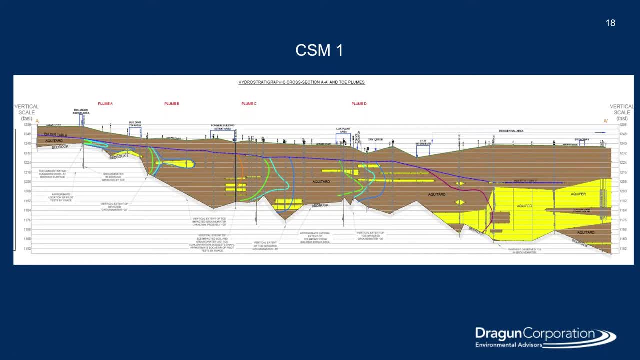 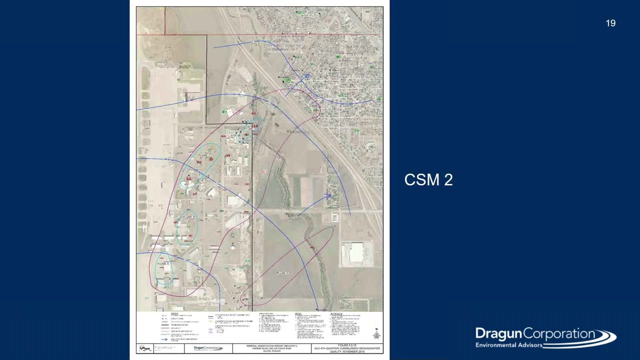 is aquifer. Those are the parts that really transmit the water readily And the white at the bottom is bedrock. And we also are showing concentrations of chemicals and the water table, in this case Slide 33, The second figure. this is a conceptual site, model part two. I suppose you could say And 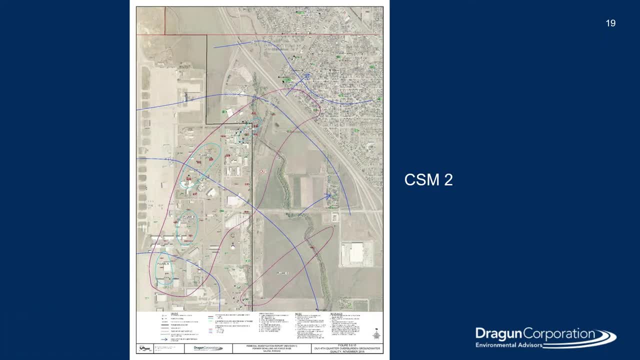 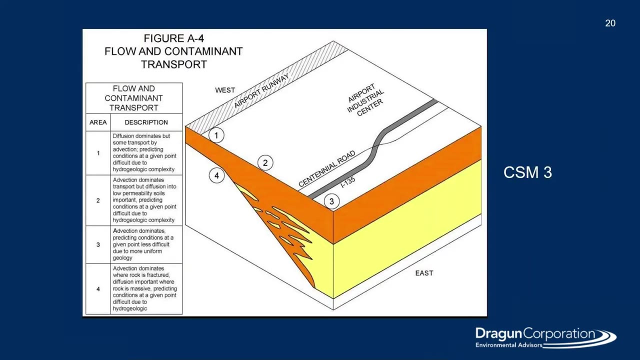 this is showing those same plumes- Slide 34. These are plumes in an aerial sense, And you can also see the groundwater contours and the groundwater flow arrows on this map- Slide 35. So that's another part of the question, And here's our very, very simplified representation. 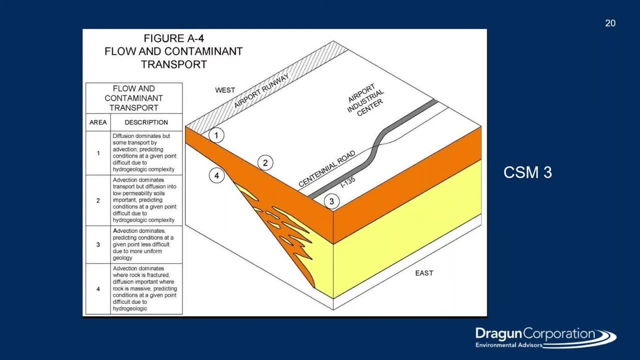 of the hydrogeology for most of the plumes And in this we're starting with very thin soil in the West- over here, Slide 35, Bedrock- and the soil progressively thins to the east And there are sand lenses that 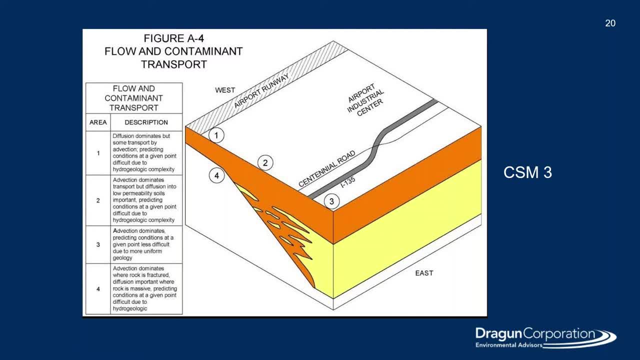 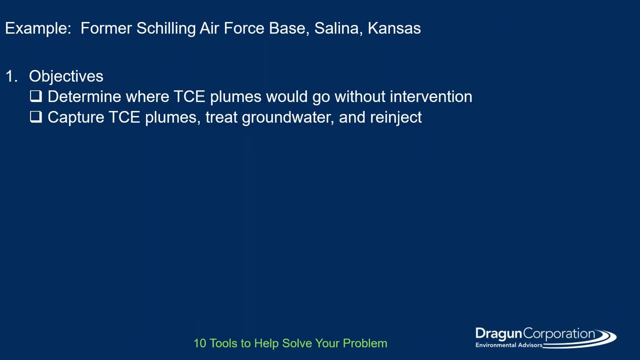 progressively get more connected, going to the east or the right, And we always keep this in mind when we're developing our computer simulation, Slide 36. So what were the examples at this? or, sorry, the objectives? The objectives at this site were to: 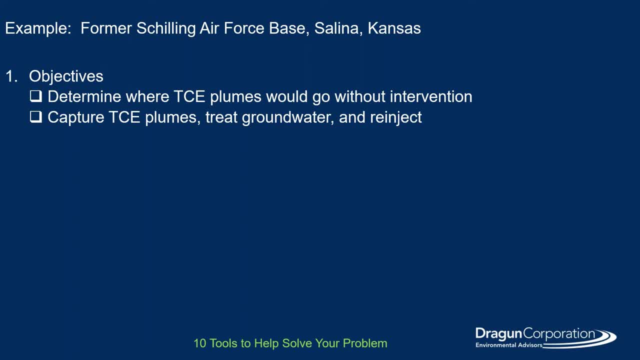 determine Slide 37, where the TCE plumes would go without intervention, If nothing were done. what would happen? And also we also use the model to help us plan to capture the plumes, to treat the groundwater and to re-inject the groundwater into the aquifers. 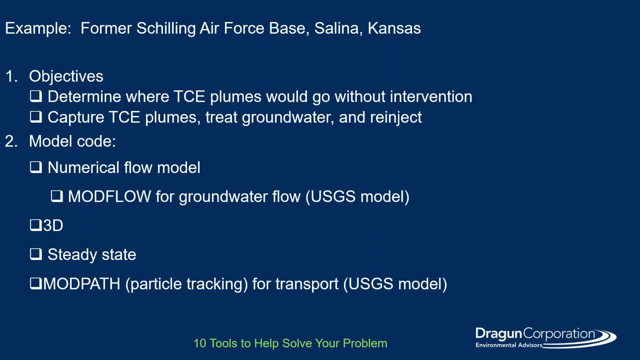 Slide 38, Slide 39. So the model code we used was a numerical flow model. because it was complex. We used mod flow for groundwater flow. It's a USGS model. We used three dimensions because we were looking at vertical and aerial changes. 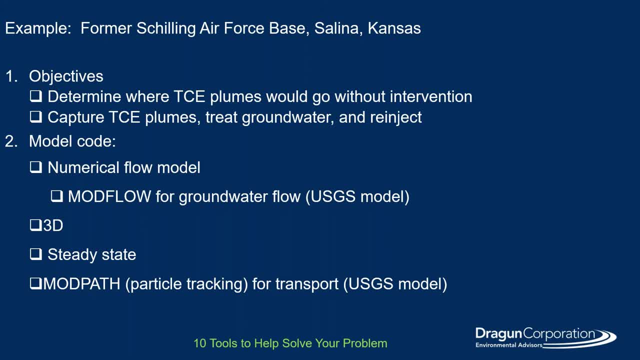 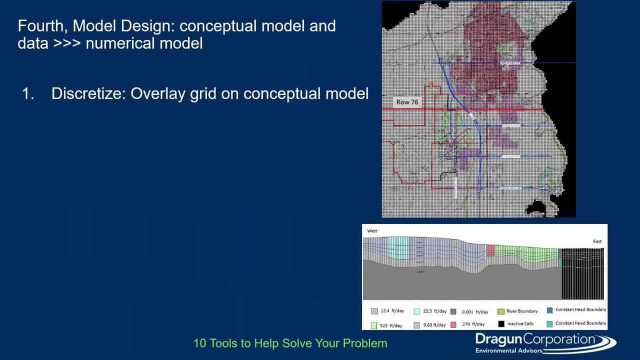 Steady state because things would not change during the running of the model And mod path for particle tracking for transport, to simplify the transport Slide 40. So next we, in the fourth step, we did the model design. The first part is to discretize the model And that means 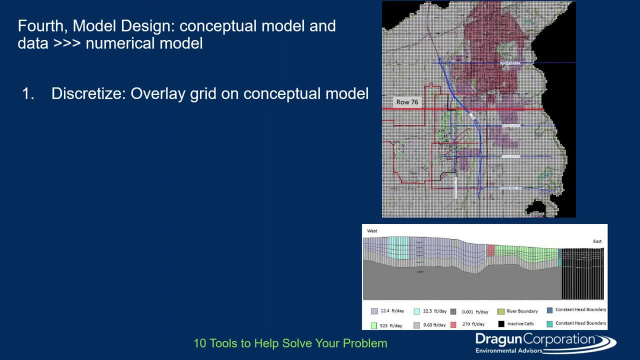 overlaying a grid on a conceptual model. There's all sorts of rules that you have to follow for this, And then you assign values to each cell in the grid, Things like hydraulic conductivity, that's how easily water can move. Slide 40. 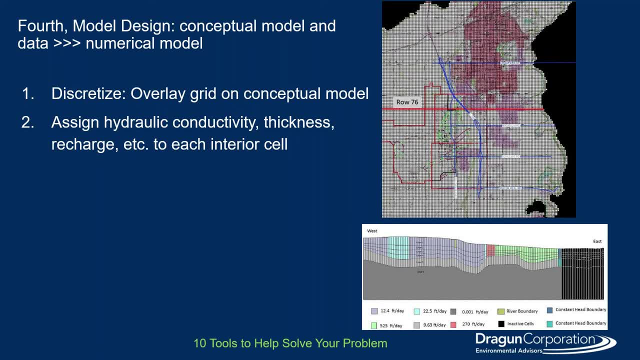 In the soil, the thickness of the cell or the soil Recharge where the water is coming in, like from precipitation, and that sort of thing to each interior cell in the model Slide 41. And then we define the boundary conditions. The boundary conditions are on the edges of 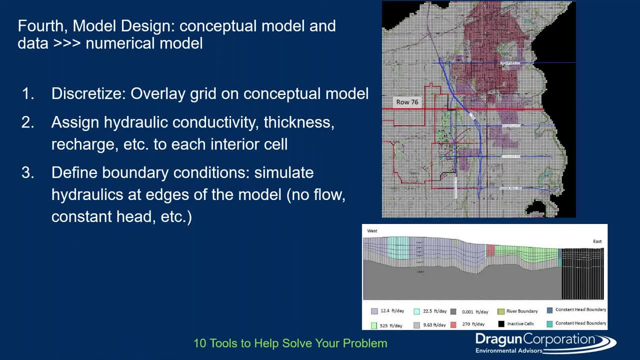 the model, And that's because we can't run the model out into infinity. In some cases we can use natural boundaries, like we see in the black, which are streams, in this case Slide 42- But in other places, like on the left side and the bottom side, we're using equations. 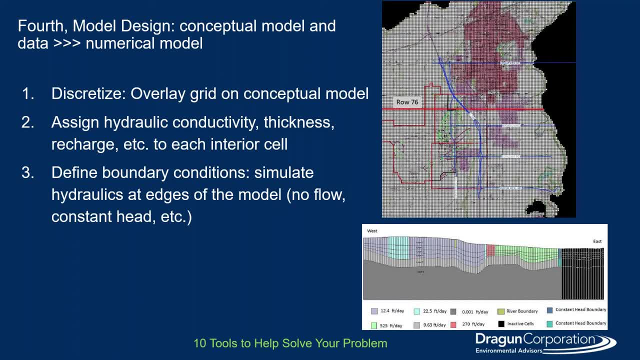 to simulate what we think the flow should be. That's a boundary condition. Slide 44: On the bottom figure you see that we have five layers above the bedrock. Slide 45, Slide 46, Slide 47 and so on. Slide 48. 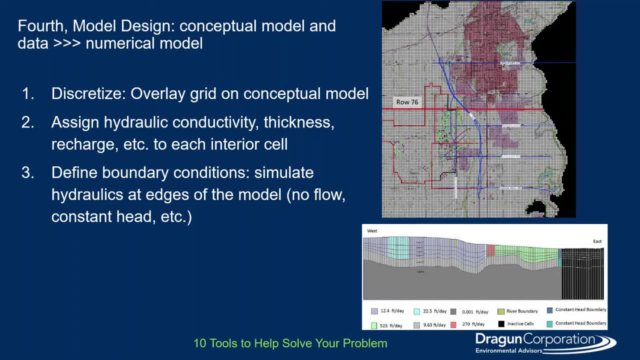 At the bottom figure, you see that we have seven layers above the bedrock, a competent bedrock in this site, and that's row 76.. So I think it's very complex. Slide 49: And then we can add things like wells that are taking water out of the system. 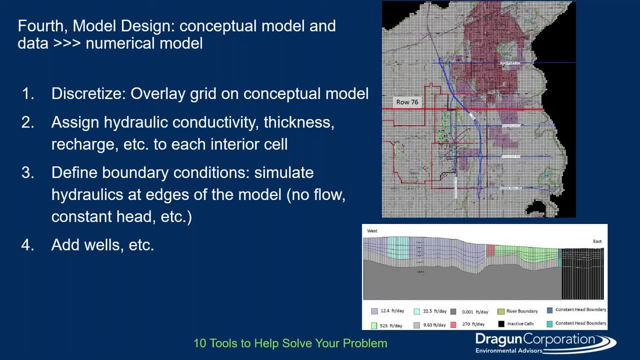 Slide 50: You can see the color coding In the cross section. the yellow are the most permeable soils. That's where the city wells are, And as you go to the left you've got less permeable soils. Slide 52: 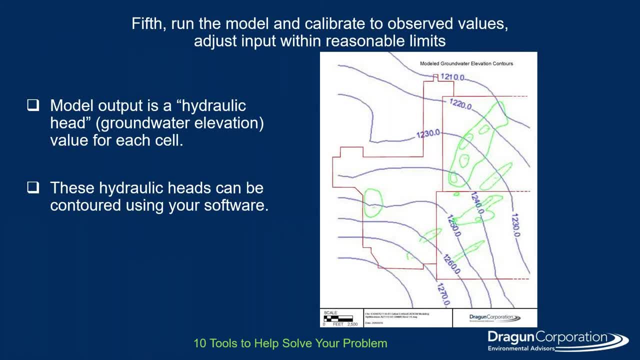 So the next step is to run the model and to calibrate, to observe values and then adjust the values within reasonable limits. Reasonable meaning: have you observed these values in your fieldwork or is it reasonable within the literature? So you can see the water level contours which we have contoured using a post processor. 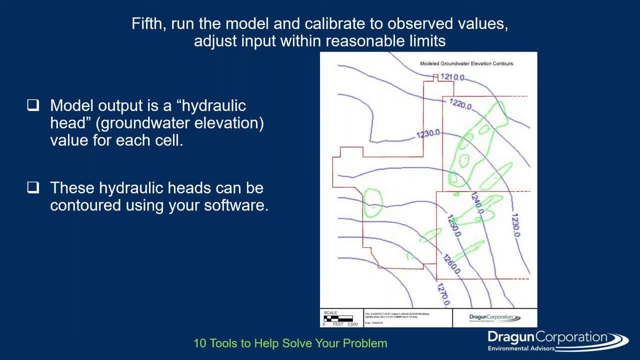 from the model And this shows the groundwater flows from the southeast to the sorry, the southwest to the northeast. We've also superimposed the observed plumes on here in the gold and yellow color, And that allows us to determine if we make sense with our groundwater flow. 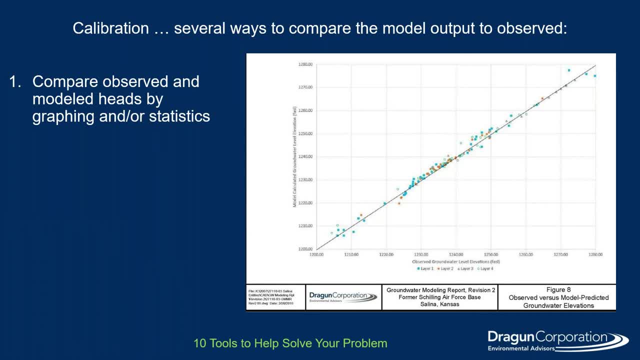 So the next step is to calibrate the model, and you can look at your calibration in several ways. This first one compares observed groundwater levels on the x-axis, the horizontal axis, to the model values at those locations On the vertical axis. the different colors represent different layers in the model. 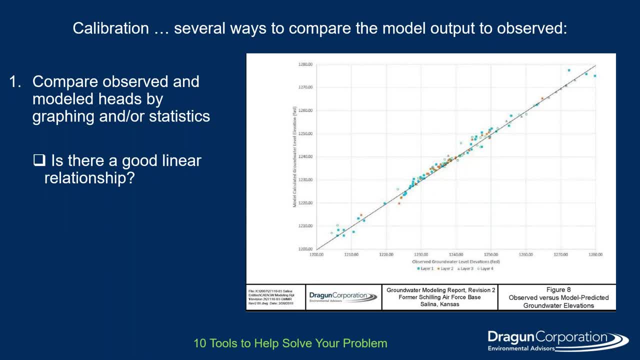 And you can see that there's a good linear relationship here. That means that it's a good calibration. What's considered a good calibration or acceptable? Well, this is a good indication. However, there are other measures of good calibration, Okay. 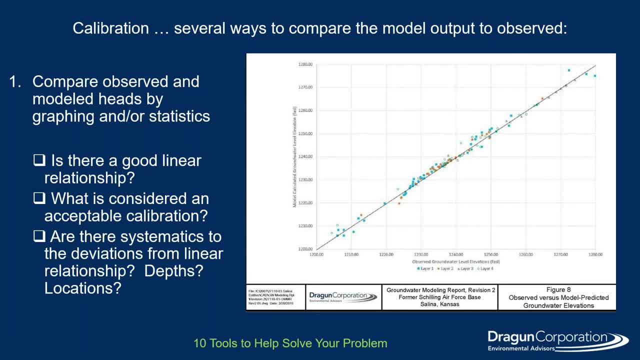 you see any systematics in the deviations from the straight line relationship, and what you want to do is look to see if if wells of a certain depth aren't represented properly, or wells in a certain area aren't represented properly, and that really is something that you should address. 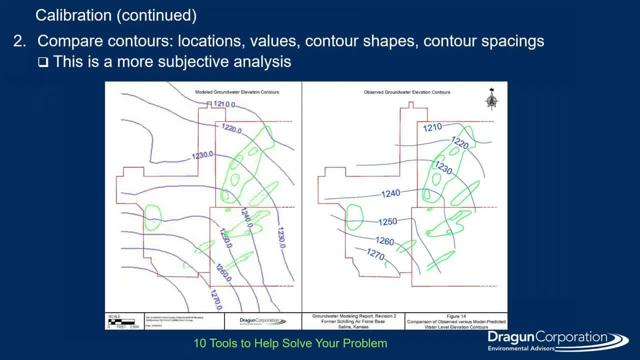 in your model. another thing that you can look at for calibration, or the locations, values, contour shapes and contour spacings. the contour spacings relate to the hydraulic gradient and that relates to transport rates. so what we've seen in this slide on the left is the model uh, contours and 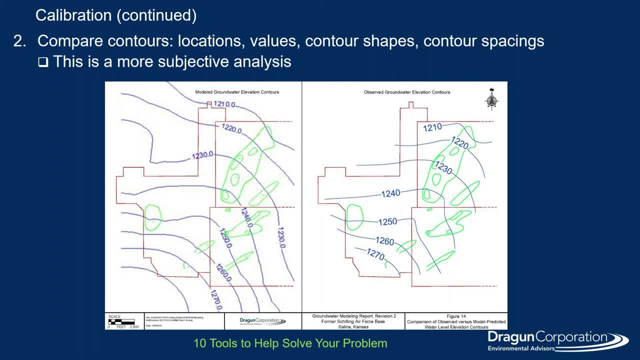 on the right you see the observed contours. again, we've got the um, the plume superimposed on this and you can see this pretty good match. the modeled contours cover a larger area than are observed because the model went beyond the area that we were had our observation wells. 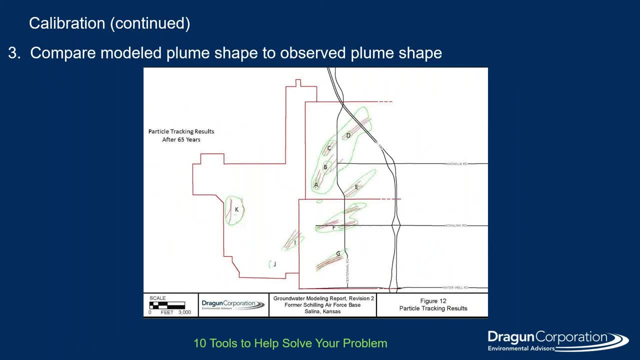 and another way to calibrate is to uh to generate plumes with your groundwater flow model, and we did this using mod path with particle tracking uh from the known source areas, knowing the approximate release dates, and then we compared that to the observed plumes. so the little red lines show uh portions of the 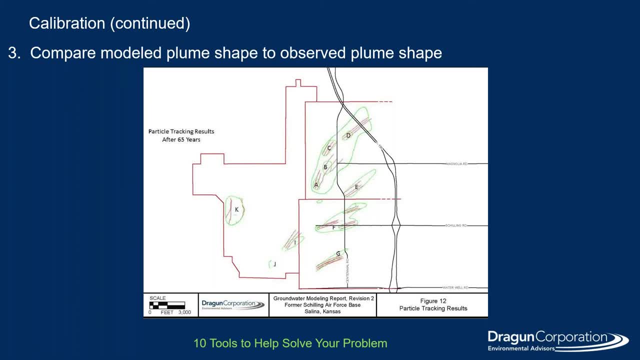 plumes- not all of them were perfect, but most of them were pretty good, and you can use what's called a retardation factor to simulate behavior of chemicals that tend to be slowed, like tce, other organic chemicals. and then we compared that to the observed plumes so that you can see that the the 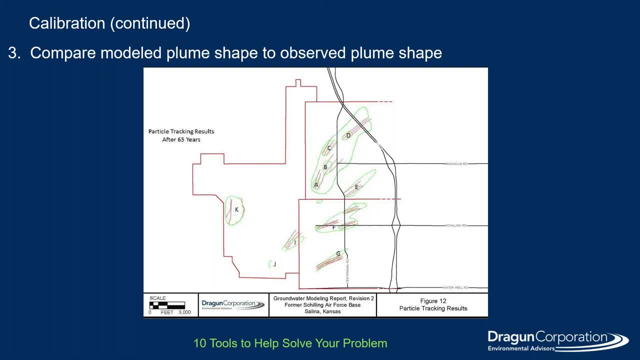 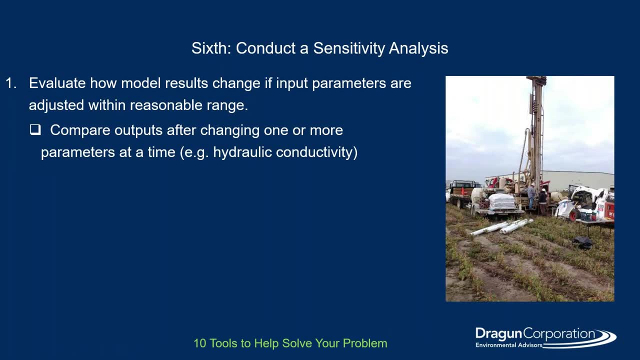 relative to the groundwater velocity. That's a subject for another webinar. So then, the next step is to conduct a sensitivity analysis. In this, we look at how sensitive is the model to specific input parameters, So we evaluate how the model results change if the input parameters are adjusted within a reasonable range. So we compare the outputs. 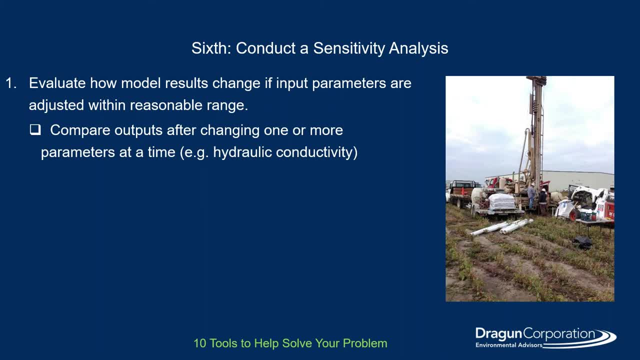 after changing one or more parameters at a time, And why does this make sense? Why do we do sensitivity analysis? Well, getting data everywhere is really it's not feasible. Getting field data is expensive, So you're looking at variations between your points. 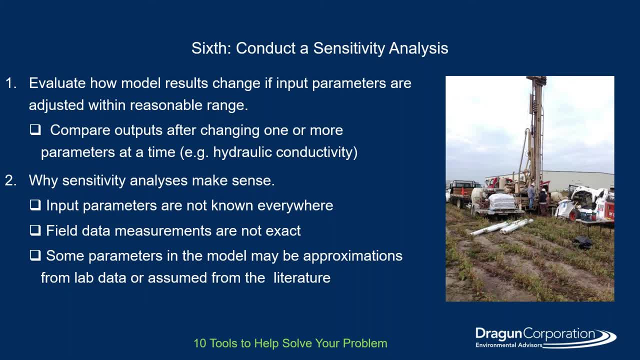 Second thing is that field data measurements are not always exactly representative of the field, that you know, that you may be off in terms of a vertical sense or lateral stance from some permeable zone, And then some parameters in the model are from approximations. 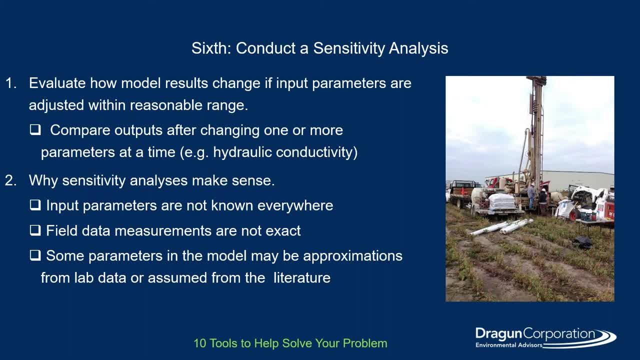 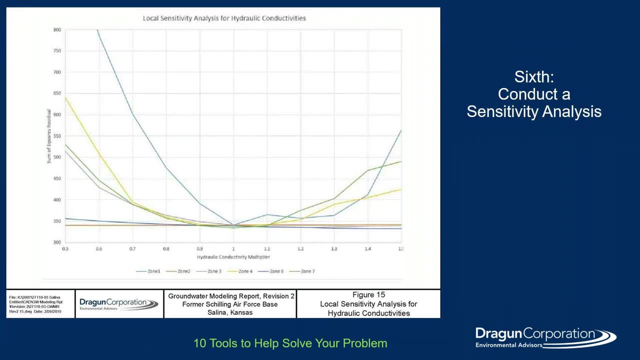 from lab data or assumed from the literature. So it makes perfect sense to use your model to and adjust the parameters to try to fit to the observed data, And this is what the output might look like. here We're looking at altering the hydraulic conductivity or permeability from the calibrated model and how that affects a statistical measurement. 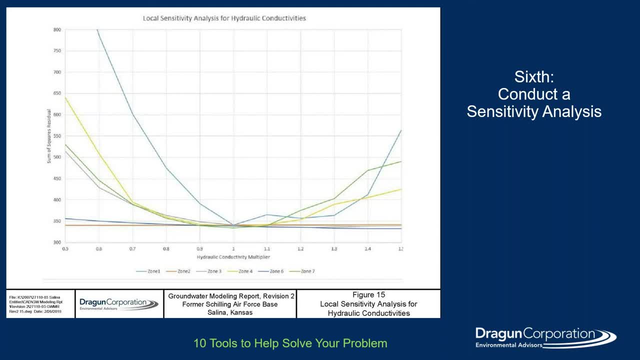 of calibration. So the permeability of one is the tip of the blue arrow. That's our calibrated model. And then on the y-axis we've got a measure of statistical calibration when we increase the hydraulic conductivity of the various layers. Each one of those lines represents an area in the model. 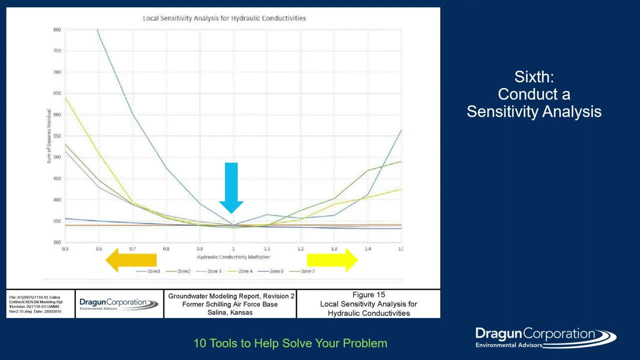 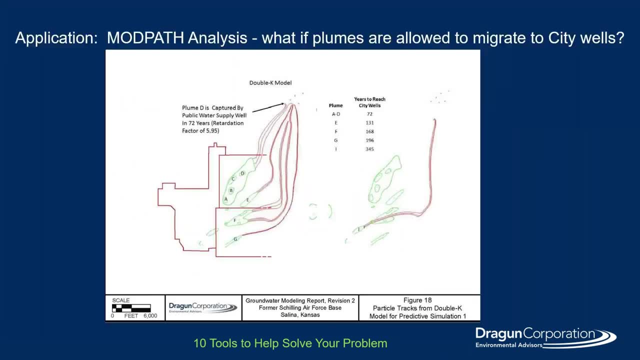 And if we decrease the hydraulic conductivity by a factor, that's what we get. So that's sensitivity analysis. So let's look at application. This is a mod flow analysis which addresses the question of what if the plumes are allowed to migrate to the city wells. 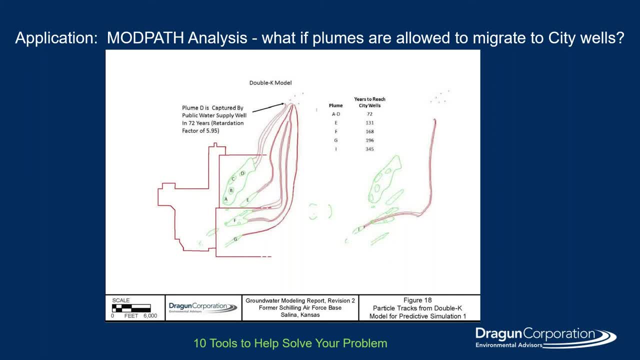 from where they are now. So what you see here is using ModPath to follow the plumes. Those are the red lines that go off to the top right, which are the city wells. that are the city wells, And the diagram on the right is just taking one of the plumes that we that kind of overlap the. 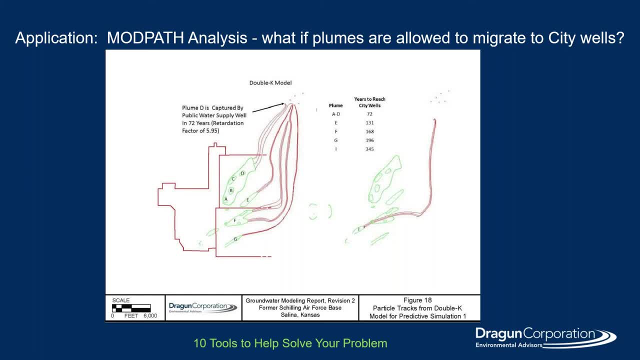 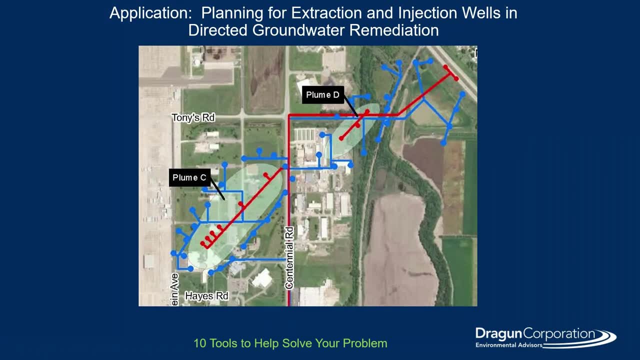 other one. So we just wanted to look at that separately. And then another application is in our remediation design. We use the model to help us plan what we call directed groundwater remediation of dissolved plumes. So you can see plume D and plume C. These 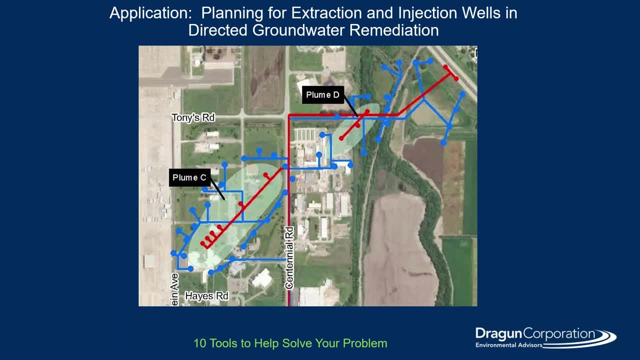 are. the slabs are two of the highest concentration plumes that need to be dealt with. the red dots are extraction wells that we propose that contain and the the plume meaning they won't let it go further. then they extract or obtain the impacted groundwater. that impacted groundwater is. 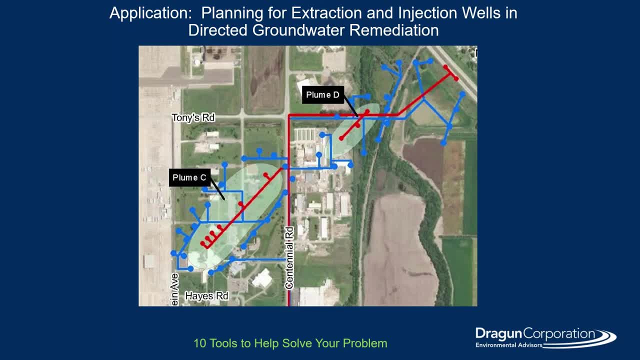 remediated above ground and we also add amendments to it. that's the plan. and then the plan is to re-inject the treated amended water in the blue dots, to force the impacted water to the extraction wells- the red dots- and to hurry up the remediation, and then we can move the wells around. 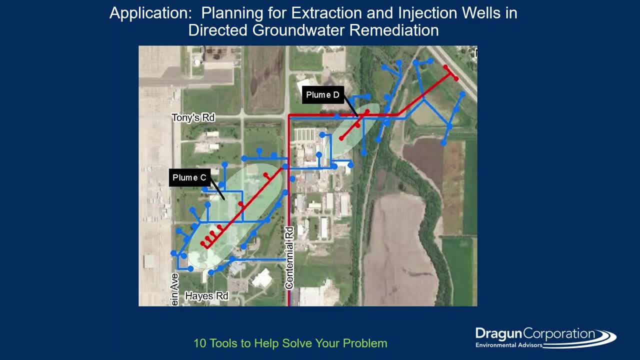 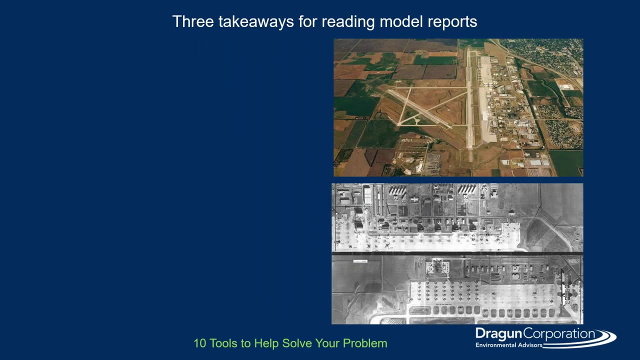 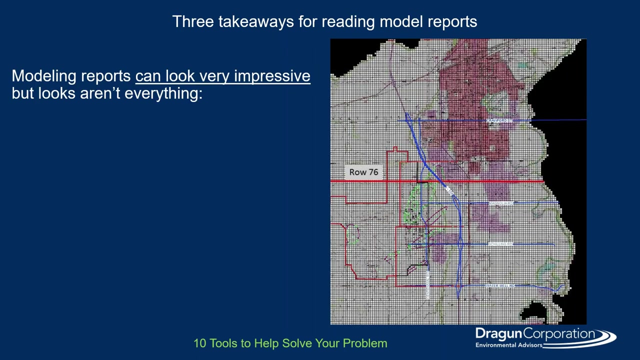 with time to optimize the remediation time. so that's what we plan to use the wells for and this is one uh iteration of that planning sequence. so three takeaways from reading modeling reports. overall modeling reports can look very impressive, but looks aren't everything. you have to make sure that the model